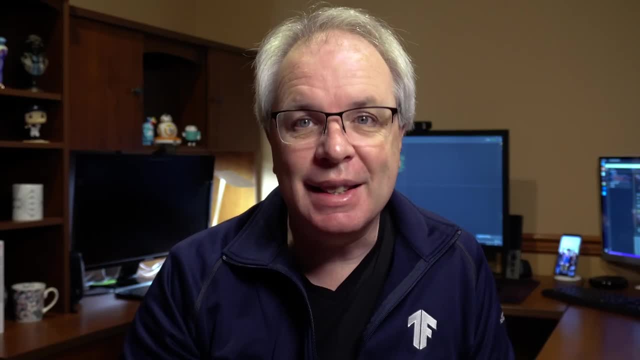 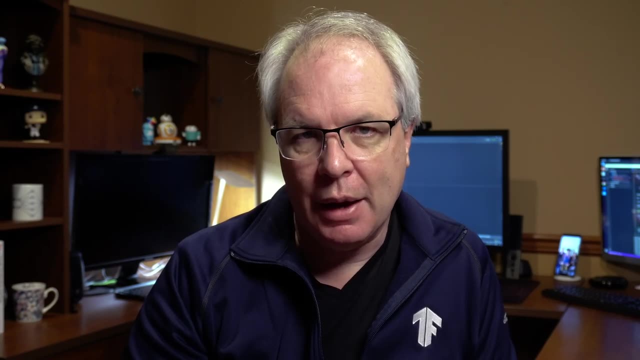 we get an AI to write poetry? Well, the answer to this is yes, And over the next few videos, I'll show you a simple example on how you can achieve this. Before we can do that, though, an important concept that you'll need to understand is: 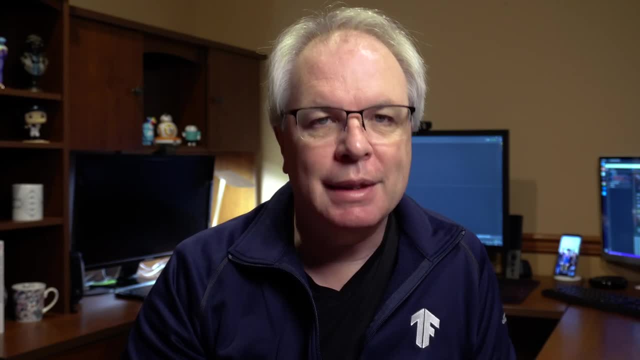 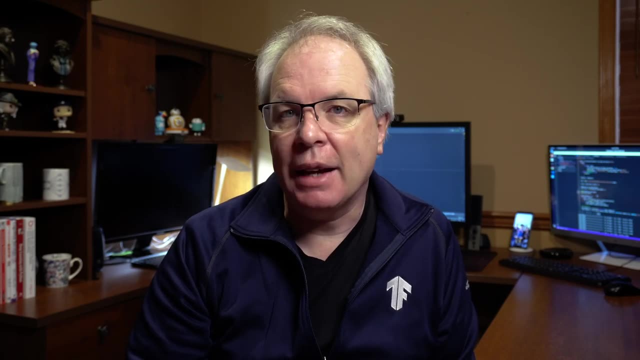 recurrent neural networks. This type of neural network takes the sequence of data into account when it's learning. So, for example, in the case of a classifier for text that we just saw, the order in which the words appear in the sentence doesn't really matter. 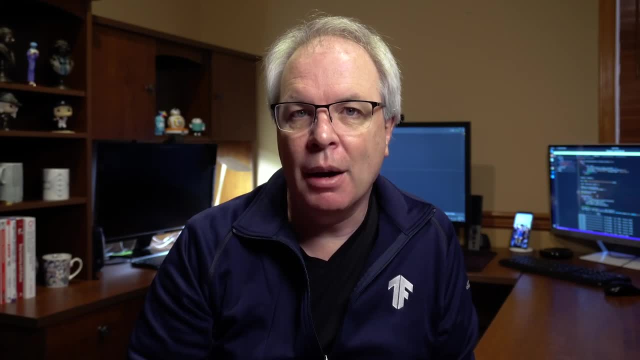 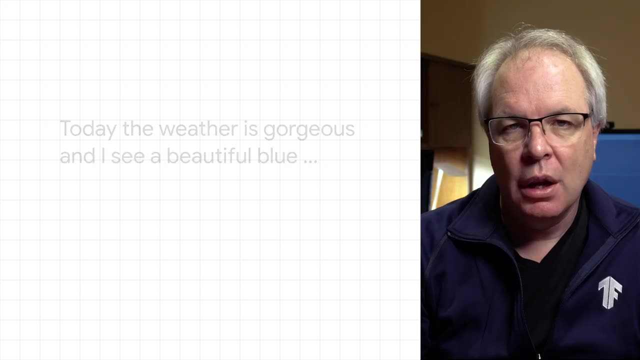 What determined the sentiment was the vector. that resulted in adding up all of the individual vectors for the individual words. The direction of that vector roughly gave us the sentiment, But if we're going to generate text, the order does matter. For example, consider this sentence: 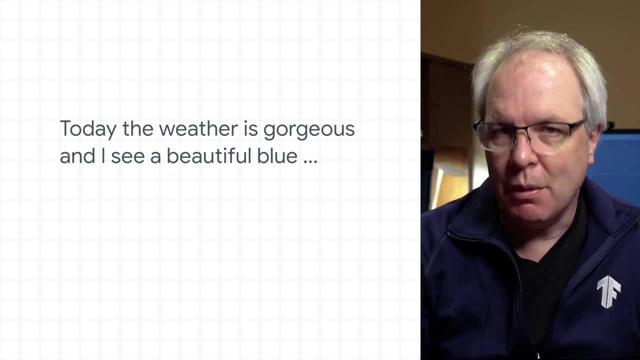 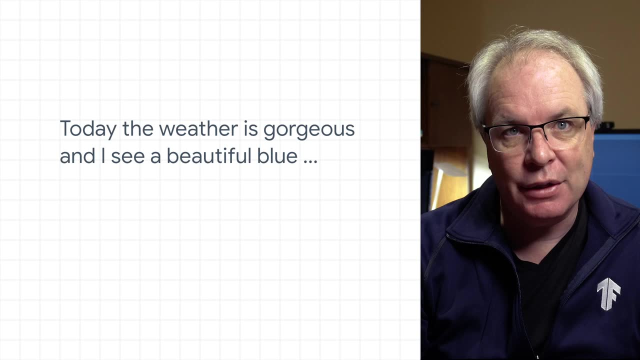 Today the weather is gorgeous and I see a beautiful blue something. If you were trying to predict the next word- and the concept of creating text really boils down to predicting the next word- you'd probably say sky, because that comes after beautiful and blue. 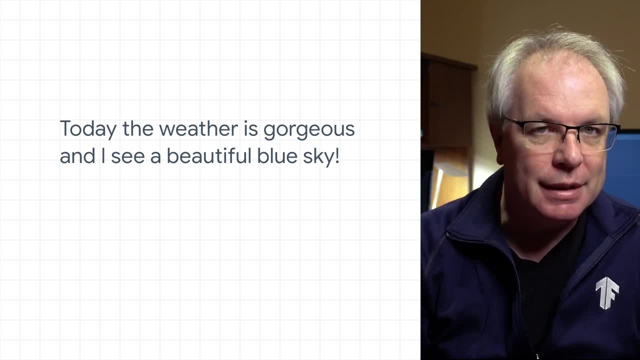 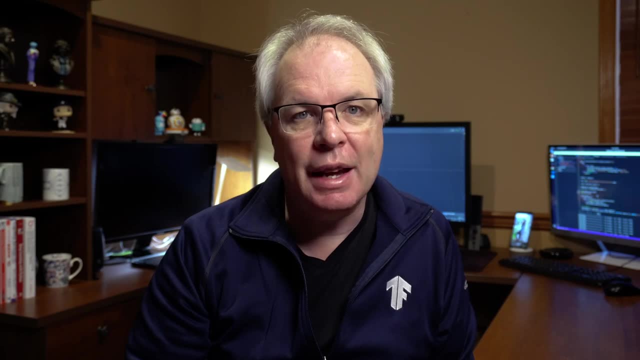 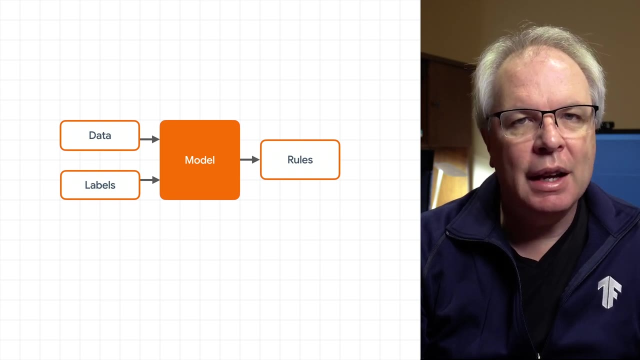 and the context is the weather, which we saw earlier in the sentence. So how do we fit this to neural networks? Let's take a look at what's involved in changing from sequence list data to sequential data. Neural networks for classification or regression tend to look like this: 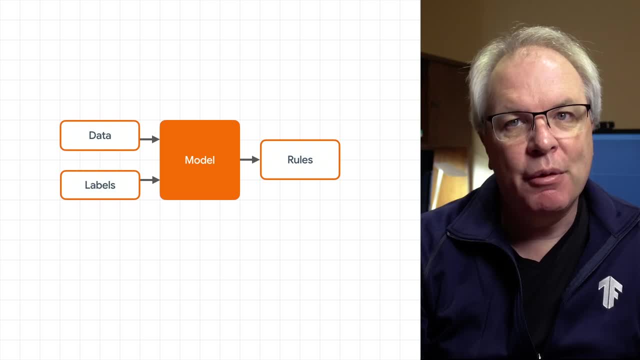 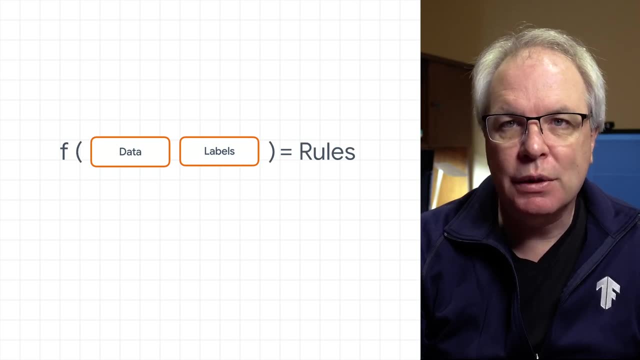 It's kind of like a function that you feed in data and labels and it infers the rules. that fits the data to the labels. But you could also express it like this: The f of data and labels equals the rules, but there's no sequence inherent in this. 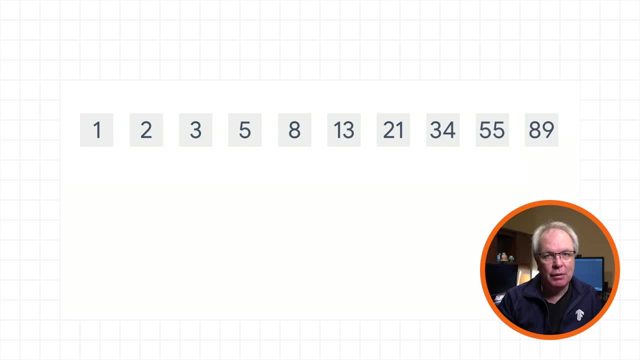 So let's take a look at some numeric sequences and explore the anatomy of them, And here's a very famous one called the Fibonacci sequence. To describe the rules that make this sequence, let's describe the numbers using a variable. So, for example, we can say n0 for the first number. 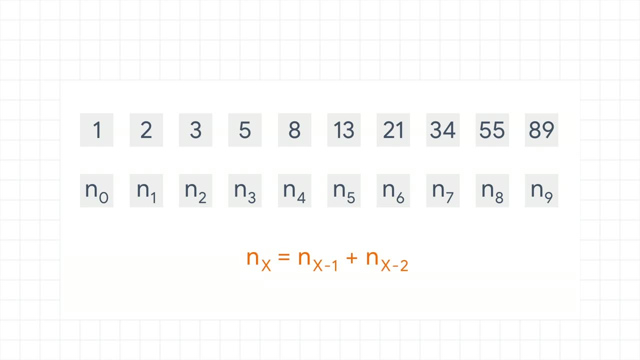 n1, for the next and so on. And the rule that then defines the number in the sequence is that any number in the sequence is the sum of the two numbers before it. So if we start with 1 and 2, the next number 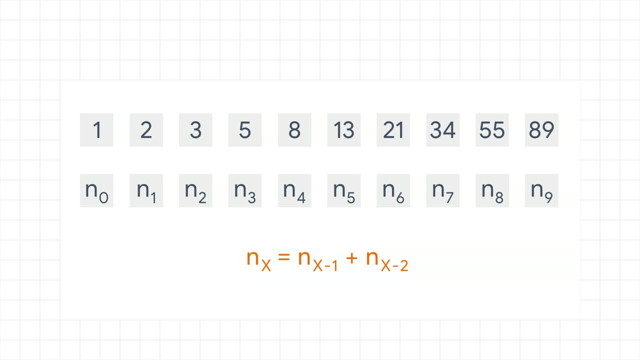 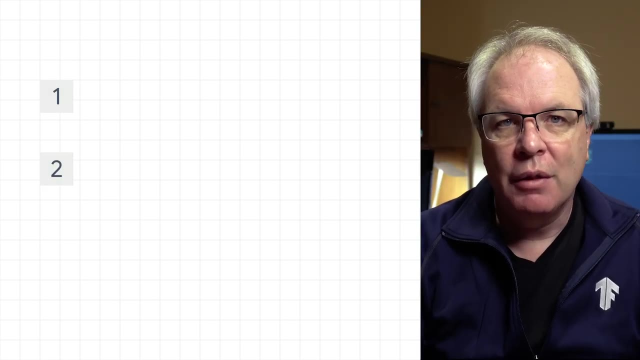 is 1 plus 2,, which is 3.. The next number is 5,, which is 2 plus 3, and so on. We could also try to visualize it like this on a computation graph: If the function is plus, we feed in 1 and 2 to get 3.. 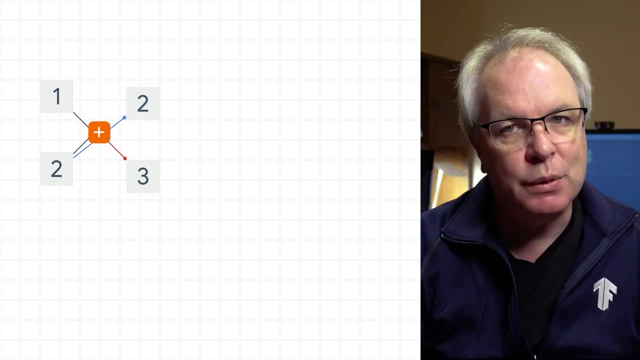 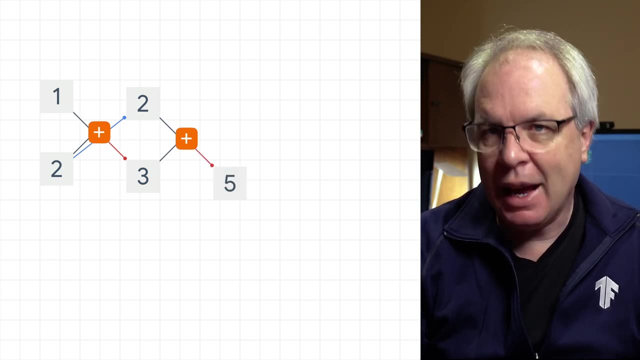 We also pass this answer and the second parameter, which in this case was 2, onto the next computation. This gives us 2 plus 3, which is 5.. This gets fed into the next computation along with the second parameter. So 5 plus 3 get added to get 8, and so on. 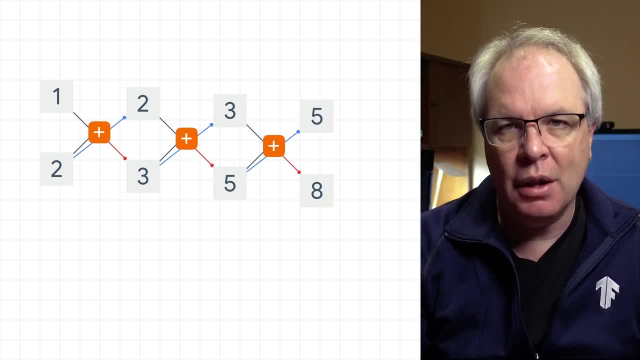 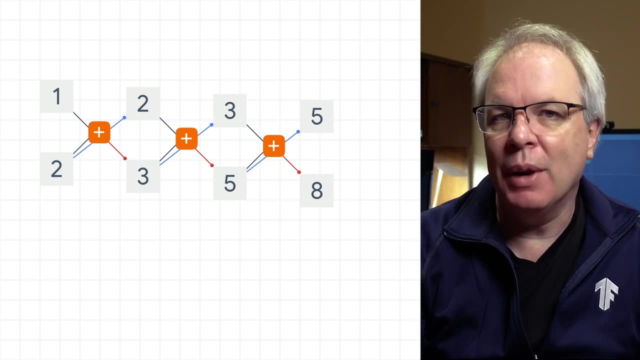 So every number is in essence contextualized into every other number. We started with 1, added it to 2 to get 3.. The 1 in the 3 still exists, And when added to 2 again, we get 5.. 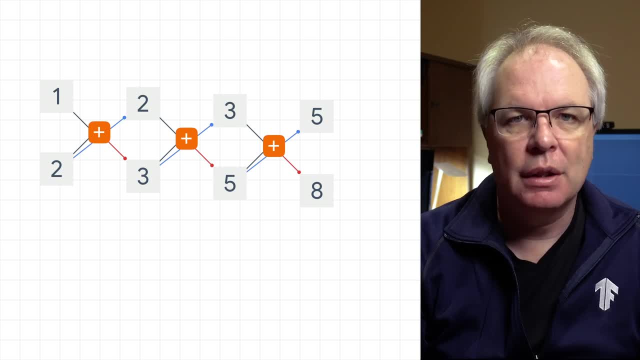 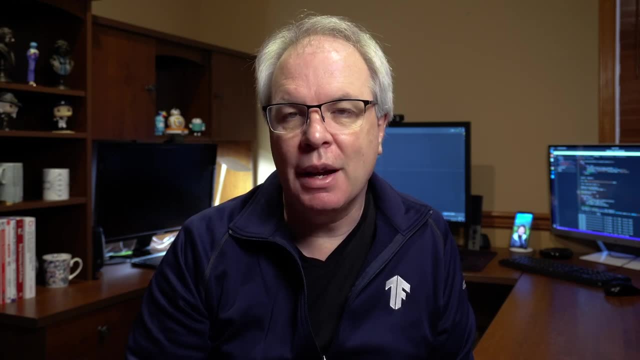 That 1 still continues to exist throughout the series. Thus a numeric value can recur. It can occur throughout the life of the series, And this is the basis of the concept of a recurrent neural network. Let's take a look at this type of network. 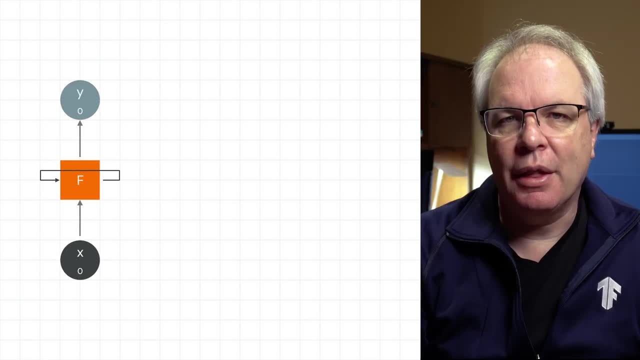 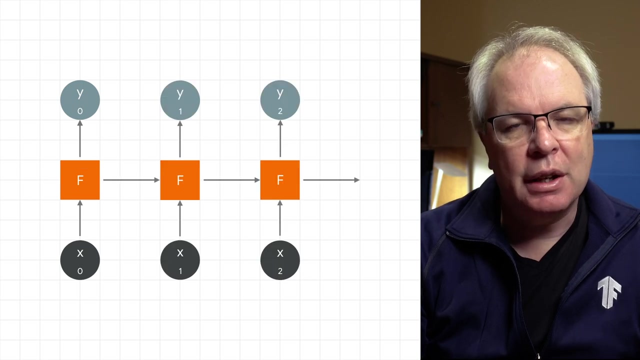 in a little more detail. Typically, a recurrent neuron is drawn like this: There's a function that gets an input value, that produces an output value. In addition to the output, it also produces another feed-forward value that gets passed to the next neuron. 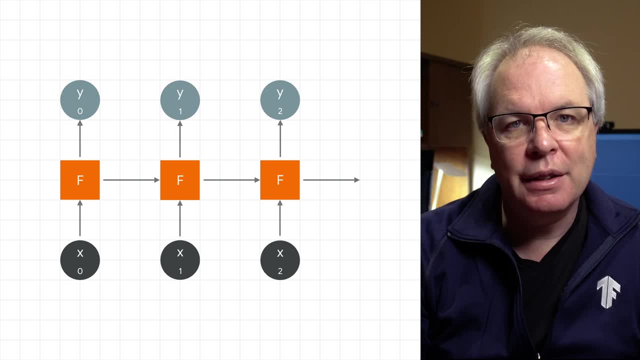 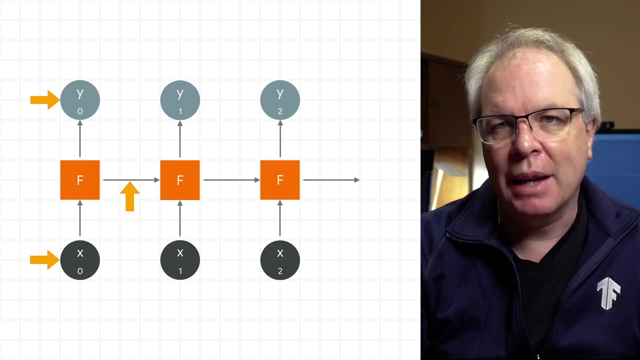 So a bunch of them together can look like this And, reading from left to right, it can feed x0 into the neuron and it calculates a result- y0, as well as a value that gets passed to the next neuron. That gets x1, along with the fed-forward value. 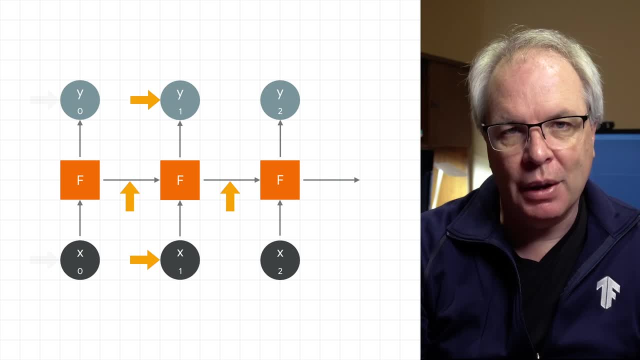 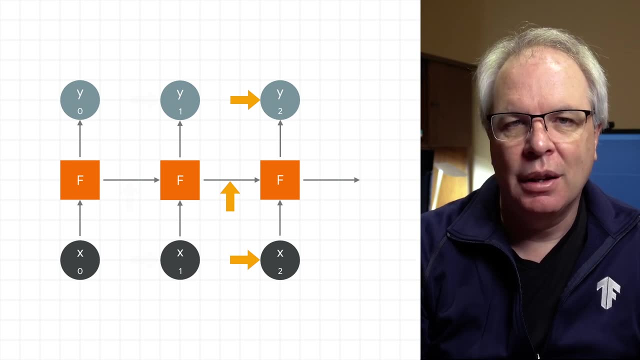 from the previous neuron and calculates y1. And its output is combined with x2 to get y2 and a feed-forward value to the next neuron, and so on. Thus sequence is encoded into the outputs a little bit like the Fibonacci sequence. 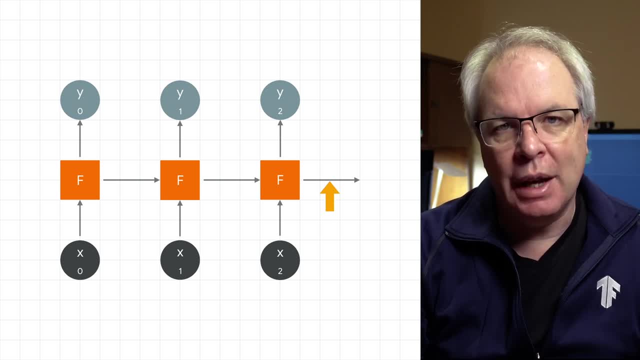 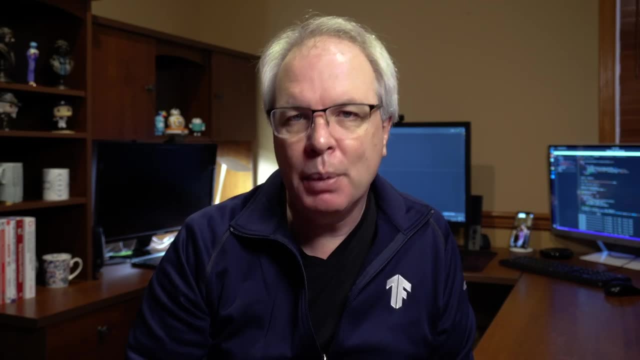 This recurrence of data, which is called the Fibonacci sequence, gives us the name recurrent neural networks. So that's all very well, And you may have seen a little catch in how this could work with natural language processing A simple RNN like the one that I've just shown.